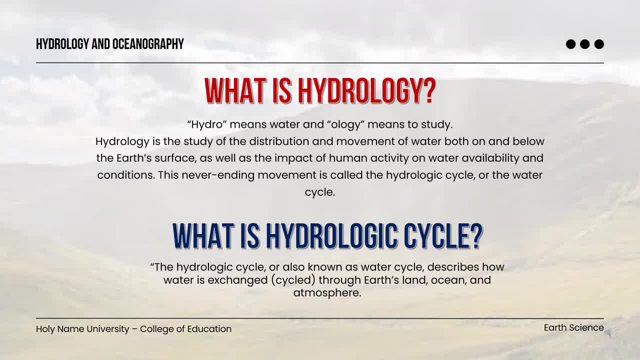 Hydrologists rely on the information of the Earth's available water. Hydrologists rely on the understanding of how water interacts with its environment, including how it moves from the Earth's surface to the atmosphere and then back to Earth. This never-ending movement is called the hydrologic cycle or the water cycle. 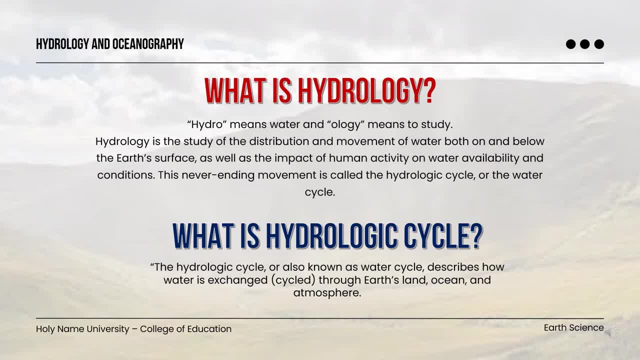 What is hydrologic cycle? The hydrologic cycle, or also known as water cycle, describes how water is exchanged through Earth's land, ocean and atmosphere. Water always exists in all three places and in many forms, as lakes and rivers, glaciers and ice sheets, oceans and seas, underground aquifers and vapor in the air and clouds. 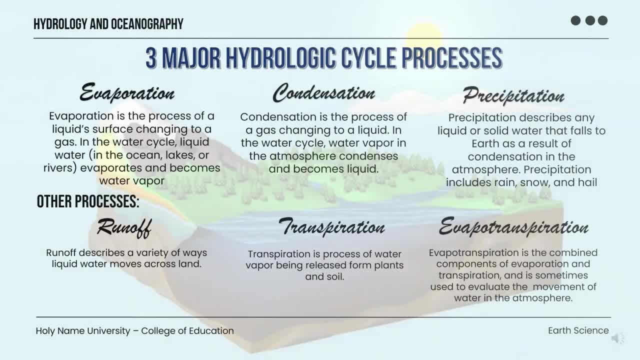 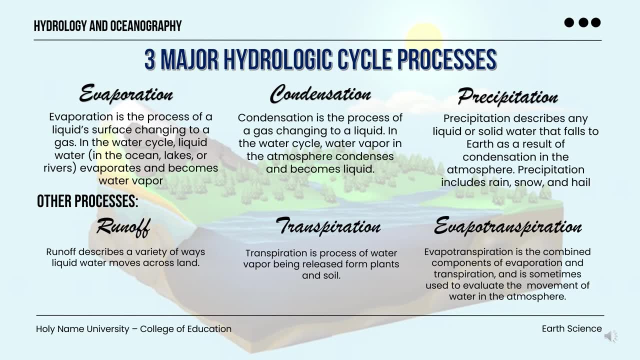 What is hydrologic cycle? The hydrologic cycle consists of three major processes: evaporation, condensation and precipitation. Evaporation: Evaporation is the process of a liquid surface changing to a gas In the water cycle. liquid water evaporates and becomes water vapor. 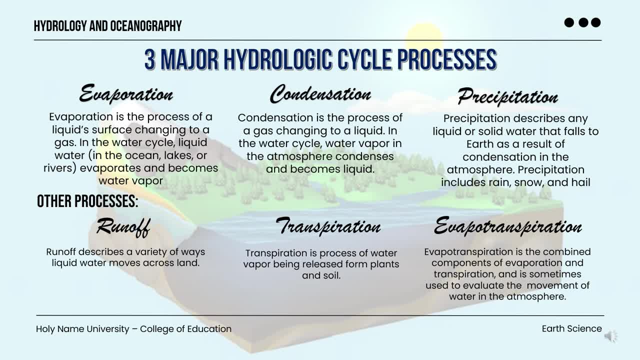 The water cycle's evaporation process is driven by the sun. As the sun interacts with liquid water on the surface of the Earth, the water becomes an invisible gas or water vapor. Evaporation is also influenced by wind temperature and the density of oxygen. 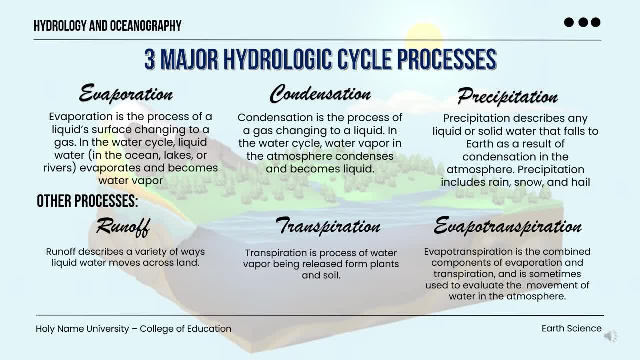 evaporation is also influenced by wind, temperature and the density of oxygen. the body of water condensation- condensation is the process of a gas changing to a liquid in the water cycle. water vapor in the atmosphere condenses and becomes liquid like evaporation. 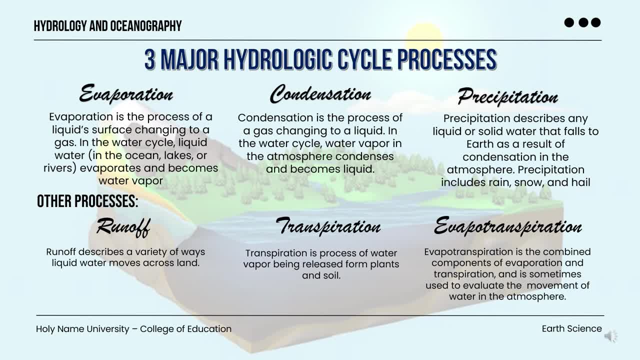 condensation is also influenced by the sun. as water vapor cools, it reaches its saturation limit or dew point. air pressure is also an important influence on the dew point of an area. precipitation precipitation describes any liquid or solid water that falls to earth as a result of condensation in the atmosphere. precipitation includes rain, snow and hail. 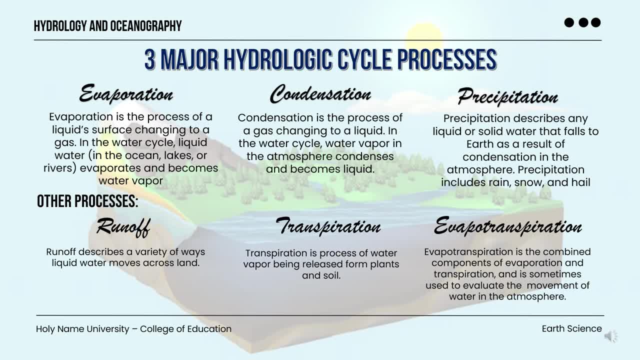 precipitation is one of many ways water is cycled from the atmosphere to the earth or ocean. evaporation, condensation and precipitation are important parts of water cycle. however, they are not the only ones. runoff runoff, for instance, describes a variety of ways liquid water moves across land. snow melt, for example, is an important type of runoff. 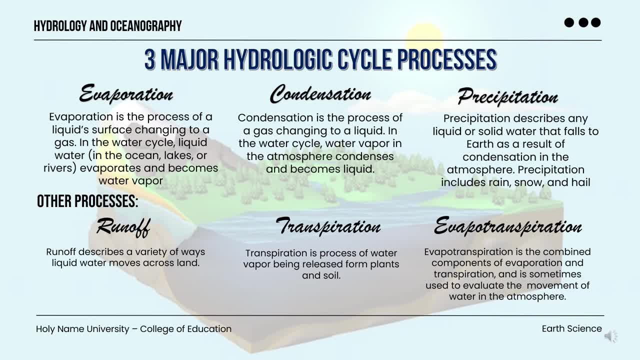 produced as snow or glaciers melt and form streams or pools. transpiration: transpiration is another form of evaporation and precipitation is another form of evaporation. the important part of the water cycle. transpiration is the process of water vapor being released from plants and soils. evapotranspiration: evapotranspiration is the 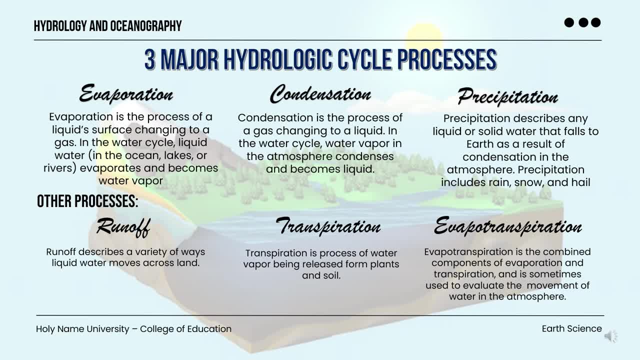 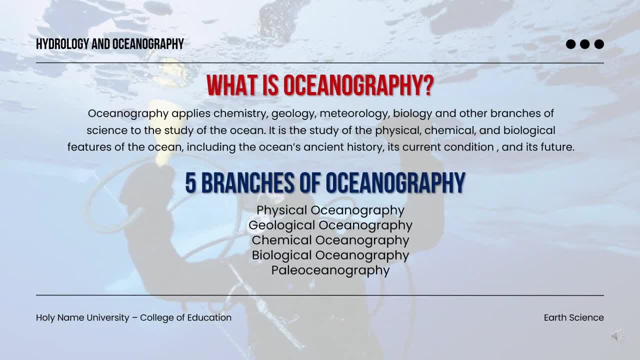 combined components of evaporation and transpiration and is sometimes used to evaluate the movement of water in the atmosphere. what is oceanography? oceanography applies chemistry, geology, meteorology, biology and other branches of science to the study of the ocean. it is the study of the physical, chemical and biological features of the ocean. 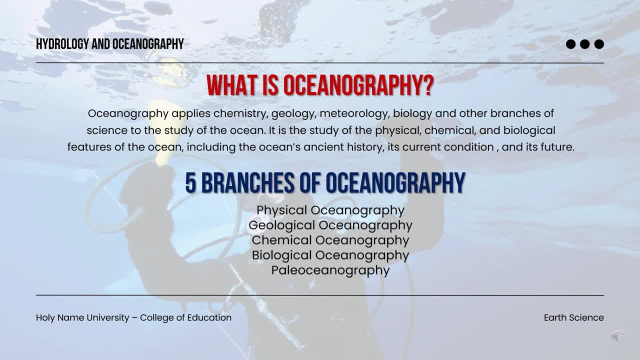 including the ocean's ancient history, its current condition and its future. in a time when the ocean is threatened by climate change and pollution, coastlines are eroding and entire species of marine life are at risk of extinction, The role of the oceanographers may be more important now than it has ever been. 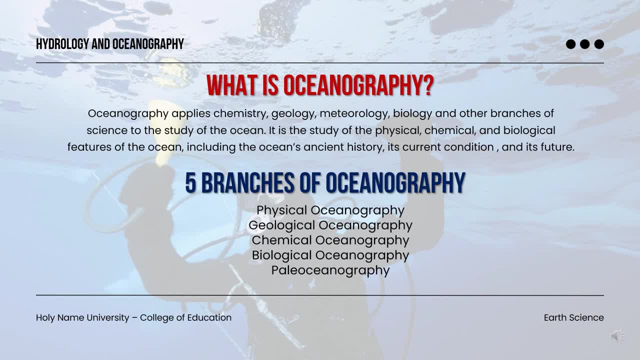 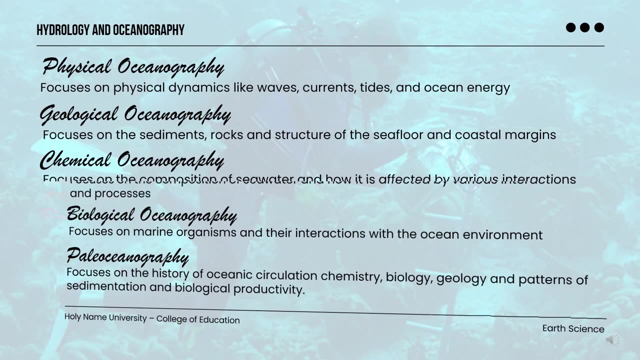 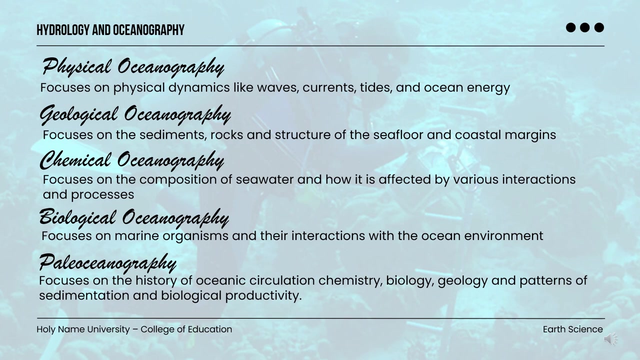 There are five branches of oceanography, namely physical oceanography, geological oceanography, chemical oceanography, biological oceanography and paleoceanography. Physical Oceanography: This focuses on physical dynamics like waves, current tides and ocean energy. 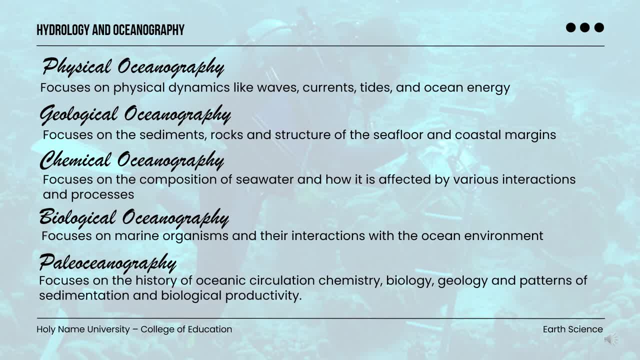 Geological Oceanography Focuses on the sediments, rocks and structure of the seafloor and coastal margins. Chemical Oceanography: It focuses on the composition of seawater and how it is affected by various interactions and processes. Biological Oceanography Focuses on marine organisms and their interactions with the ocean environment. 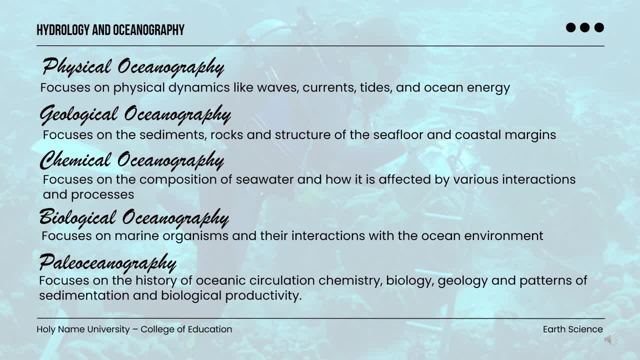 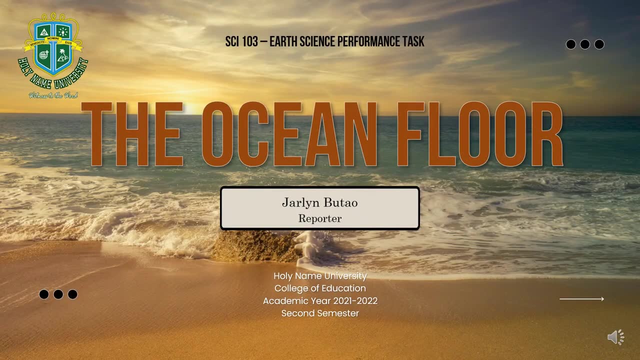 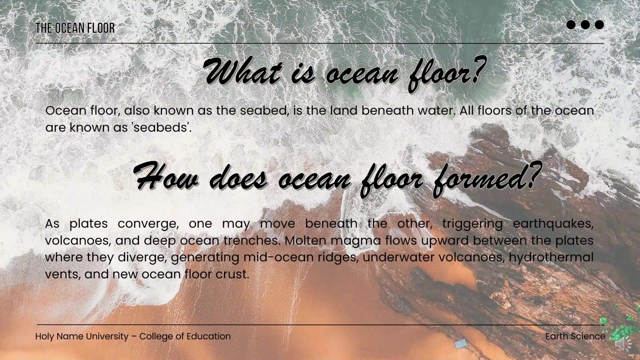 Paleoceanography. This focuses on the history of oceanic circulation, chemistry, biology, geology and patterns of sedimentation and biological productivity. The Ocean Floor: Biochemical Oceanography. What is the ocean floor? What is the ocean floor? Ocean floor, also known as the seabed, is the land beneath water. 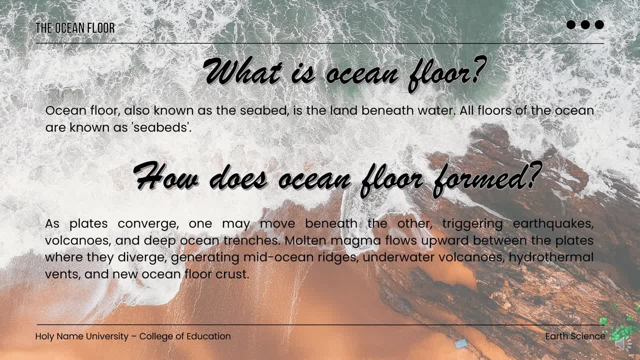 All floors of the ocean are known as seabeds. How does ocean floor form? As plates converge, one may move beneath the water, triggering earthquakes, volcanoes and deep ocean trenches. Molten magma flows on upward between the plates where they diverge, generating mid-ocean losses. MULTEN MAGMA FLOWS ON UPWARD BETWEEN THE PLATES WHERE THEY DIVERGE, GENERATING MID-OCEAN LONG, MULTIPLE PLATES. MULTEN MAGMA FLOWS ON UPWARD BETWEEN THE PLATES WHERE THEY DIVERGE, GENERATING MID-OCEAN LONG, MULTIPLE PLATES. 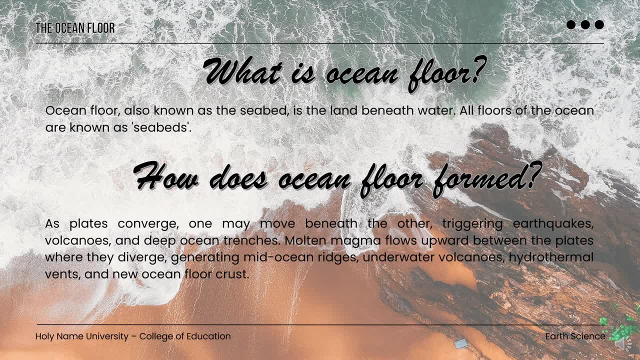 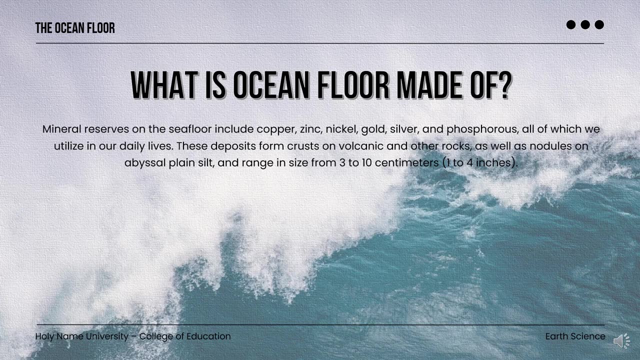 where they diverge, generating mid-ocean ridges, underwater volcanoes, hydrothermal vents and new ocean floor crust. What is ocean floor made of? Mineral reserves on the seafloor include copper, zinc, nickel, gold, silver and phosphorus- oil or which we utilize in our daily lives. 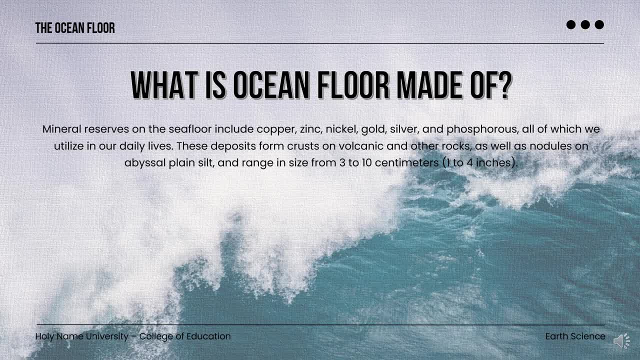 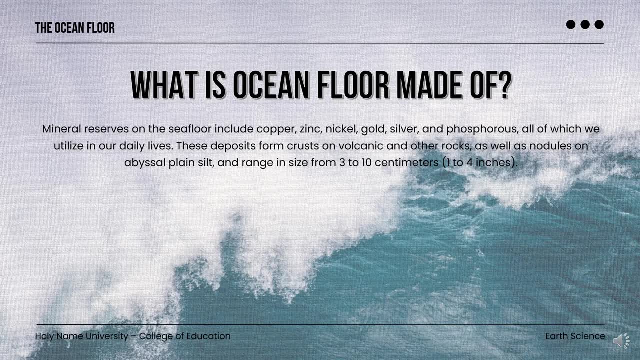 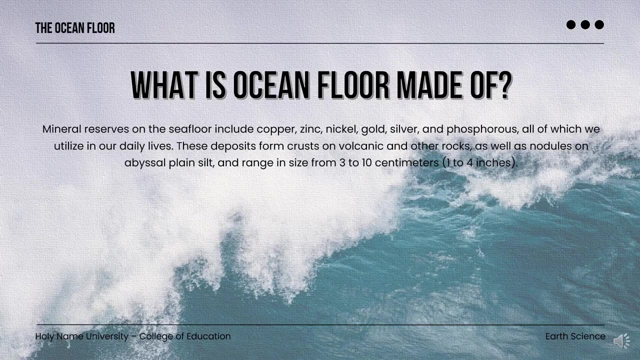 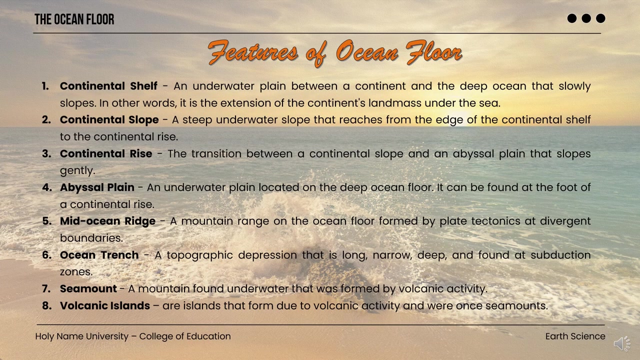 These deposits from crusts and volcanic and other rocks, as well as nodules on abyssal plains, silt, and range in size from 3 to 10 cm. 1 to 4 inches. Features of Ocean Floor. First Continental Shelf. 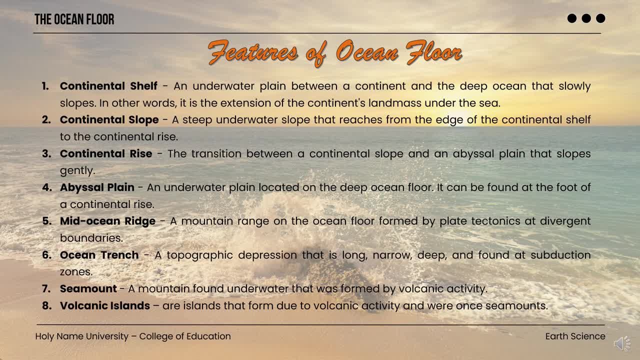 An underwater plain between a continent and the deep ocean. It is the extension of the continent's landmass at the sea. Second Continental Slope: A slip underwater slope that reaches from the edge of the continental shelf to the continental rise. Third Continental Rise. 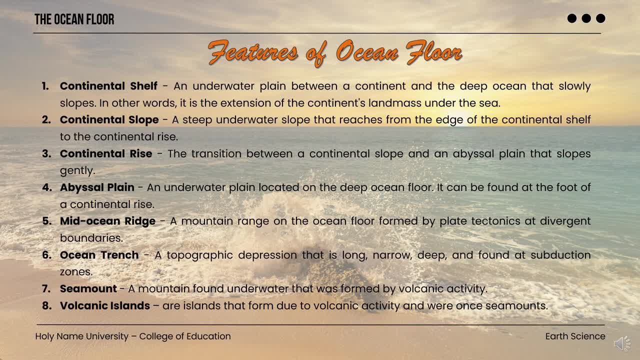 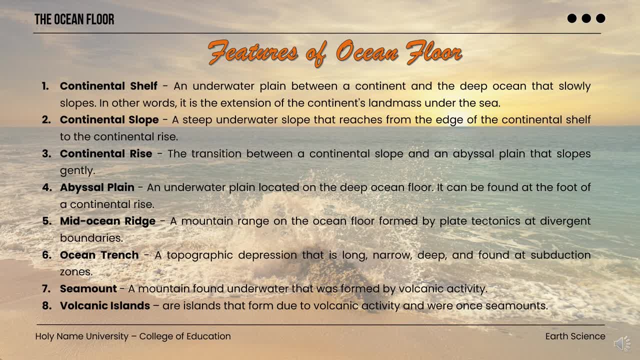 It can be found on the seafloor, The foot of a continental rise. Mid-ocean ridge, A mountain range of the ocean floor formed by plate tectonics at divergent boundaries. Ocean trench, A topographic depression that is long, knurled deep and found subduction zarus. 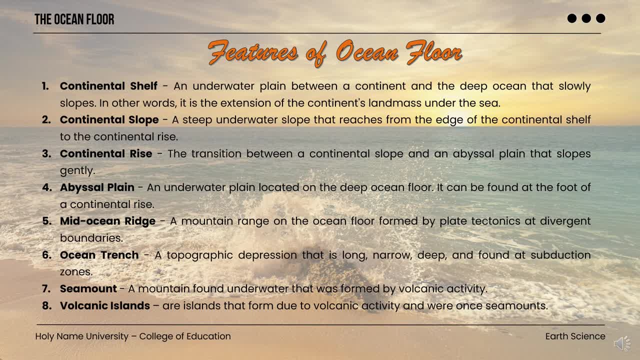 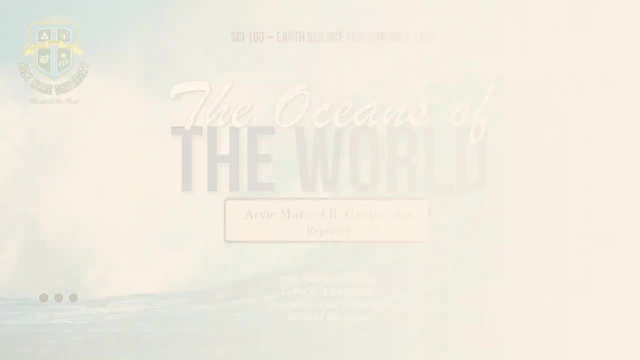 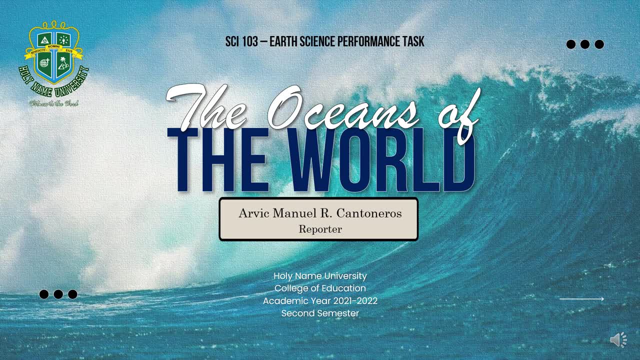 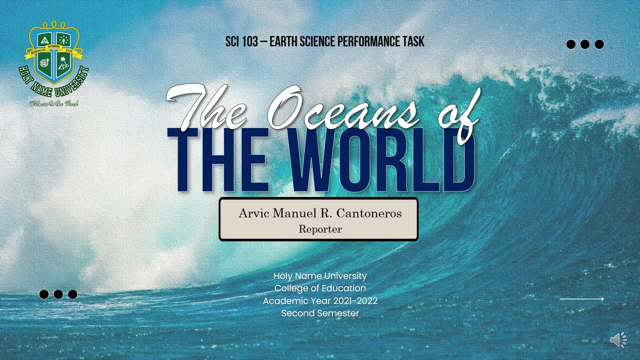 Hello and good afternoon everyone. Just earlier we have learned from Ms Buligaw about the basics and the definitions of hydrology and oceanography. In addition to that, Ms Butaw also discussed about the ocean floor, how it is formed, its 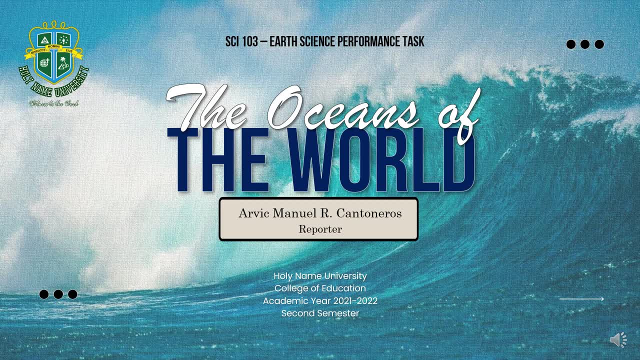 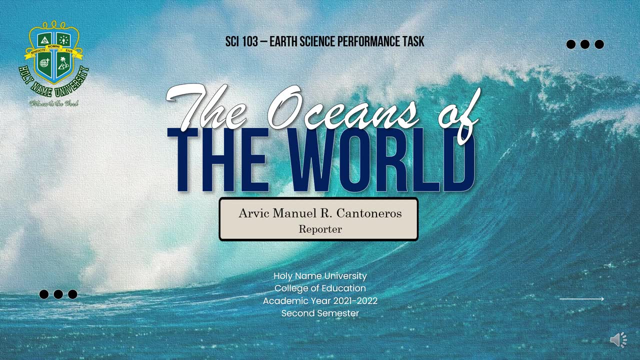 features and some other details about it. So at this juncture, allow me to introduce myself first. I am Arvik Manuel R Cantoneiros, I am the third reporter from this group and I am going to talk about the oceans of the world. 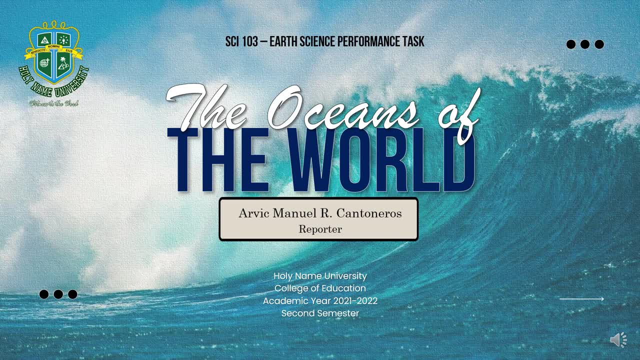 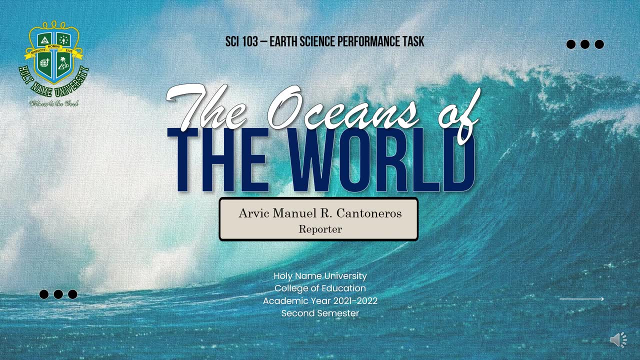 So, when we talk about oceans, what comes into your mind, or the idea that pops up into your head when you hear that specific word? Alright, so I believe that everyone of you here would actually say that an ocean is a large body of saltwater that surrounds the 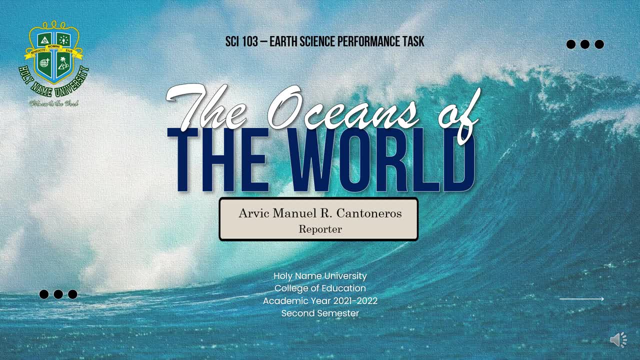 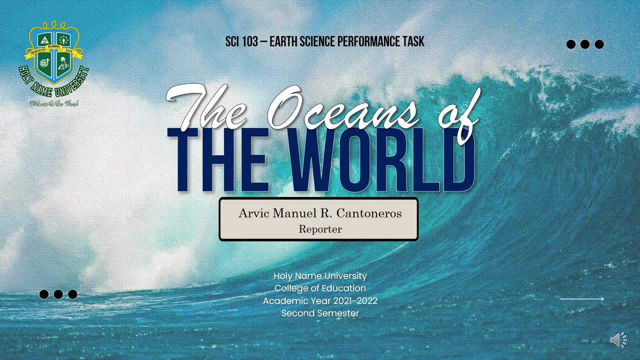 continents, which is actually true. that is correct. So for this whole presentation, we will be talking about the oceans, the definition of ocean and the five major regions or the five major oceans of the world. So I hope that everyone is ready. 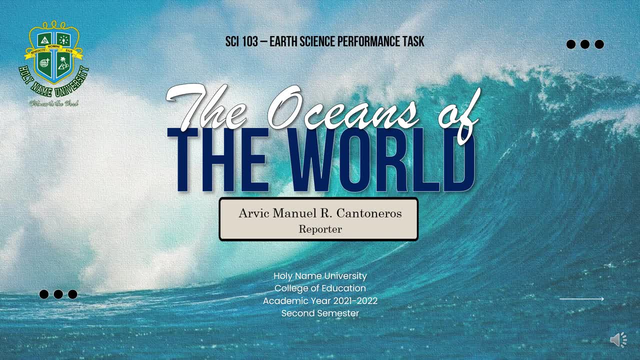 I hope that you have your pens and notebooks ready. I hope that you have your pens and notebooks ready. So I hope that you have your pens and notebooks right there with you right now, because we will be having a quiz after this entire presentation. 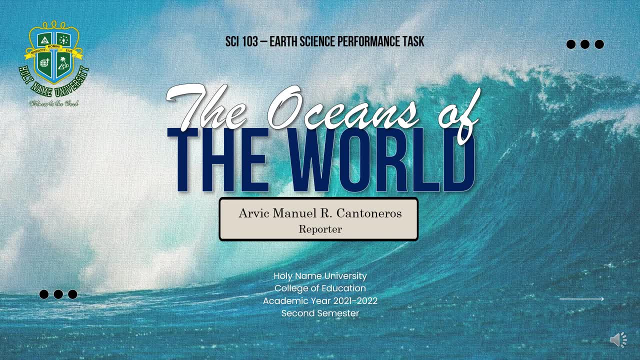 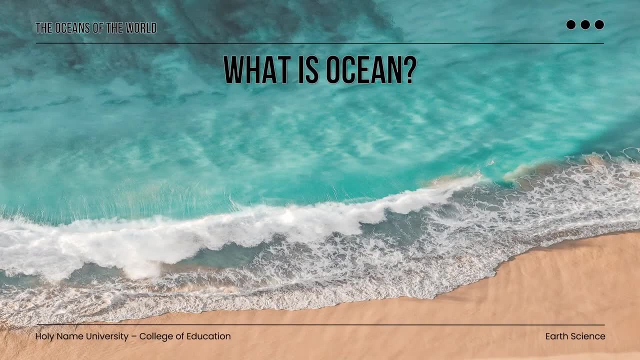 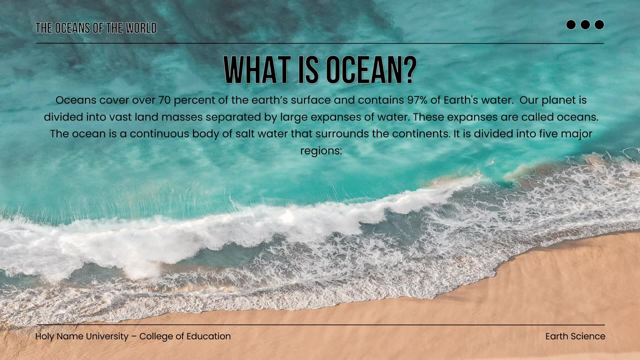 So are you ready? Let us now proceed to our proper discussion. So what the ocean really is. Oceans cover over seventy percent of the earth's surface and it contains ninety-seven percent of earth's water. Our planet is divided into three parts. 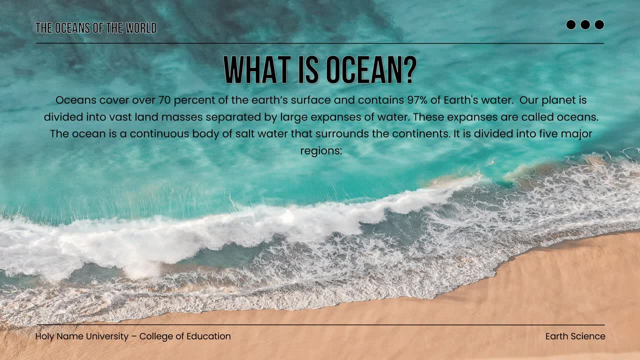 The Earth is divided in two parts. Where is the Earth? Where is the Earth? vast landmasses separated by large expanses of water. so if we are going to look at a global map, we can observe that it has a color green and color blue. that 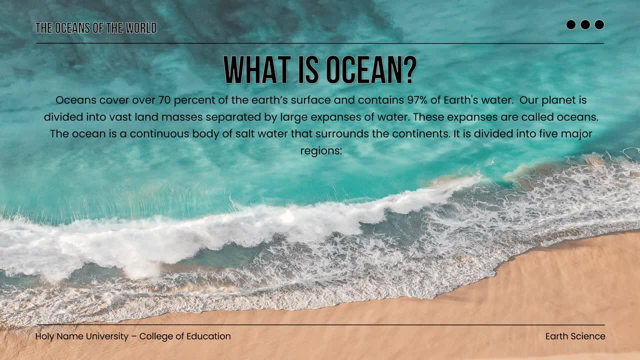 green portion is the land masses and the blue one, which surrounds the green one, is the water, or our oceans, so that expanses are called oceans. the ocean is a continuous body of salt water that surrounds the continents. so if this actually divided into five major regions, we have first Pacific Atlantic Indian. 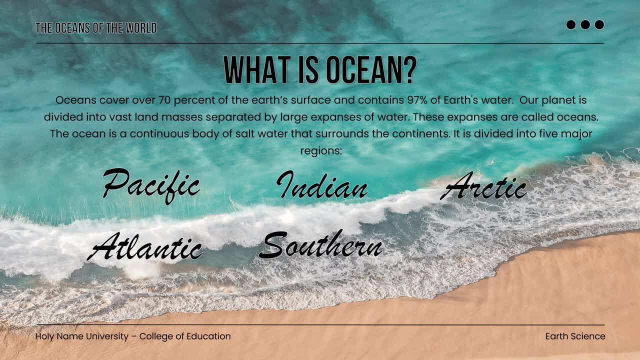 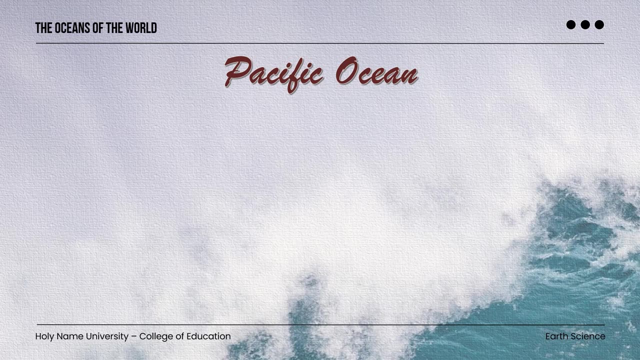 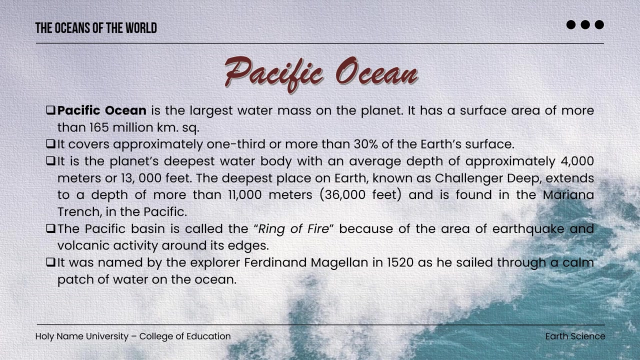 Southern and Arctic respectively. so for this presentation we will be talking about these regions one by one. so let us first about Pacific Ocean. Pacific Ocean is the largest watermass in the planet. it has a surface area of more than 165 million kilometers squared. it covers approximately one-third, or more than 30 percent, of the Earth's surface. so 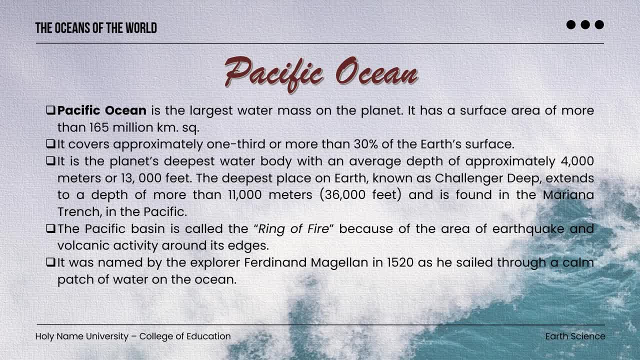 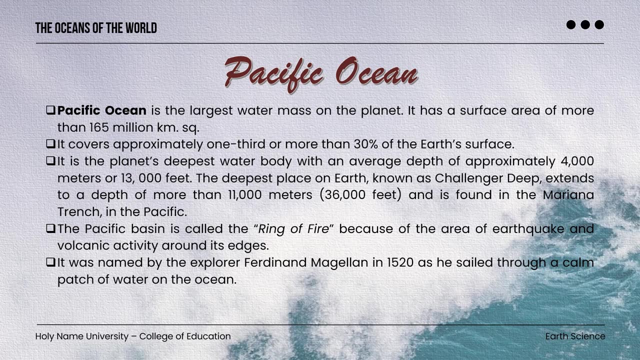 imagine the Pacific Ocean and, by the way, the Philippines- and I know that you already know about this- Philippines- is located in the Pacific. it is the planet's deepest water body, with an average depth of approximately 4,000 meters, or 13,000 feet. the deepest place on earth, known as Challenger Deep. 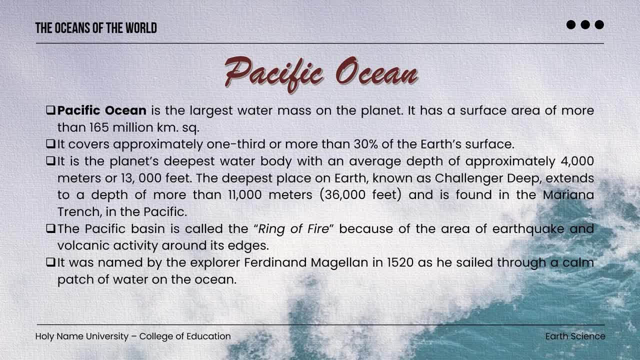 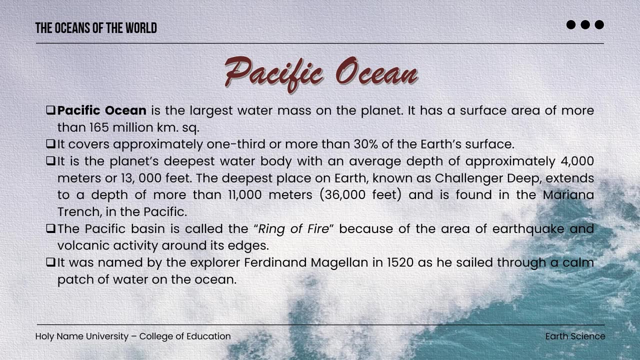 extends to a depth of more than 11,000 meters or 36,000 feet, and is found in the Mariana Trench in the Pacific. the Pacific Basin is called the Ring of Fire because of the area of earthquake and volcanic activity around its edges. it was named by the explorer Ferdinand Magellan in 1520 as 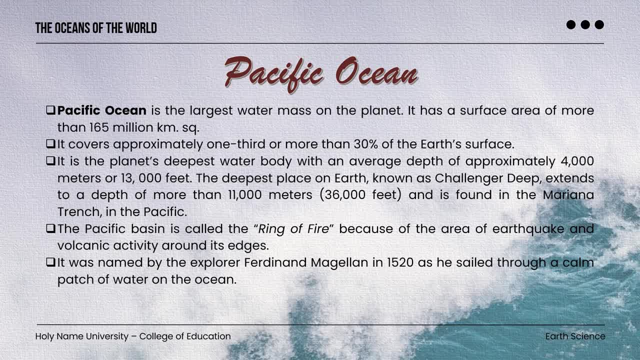 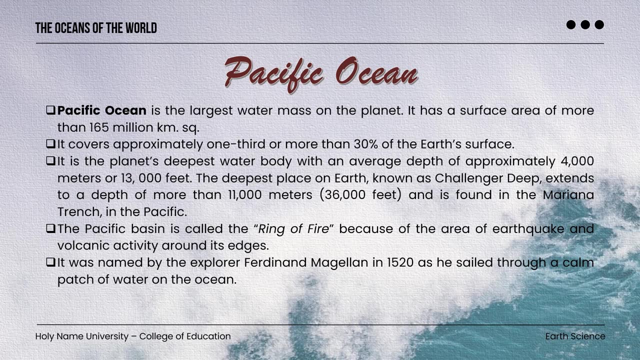 he sailed through a calm patch of water on the ocean. so this is a very interesting information about the Pacific Ocean. I I guess because accordingly Ferdinand Magellan named this ocean Pacific- because as he was sailing through, sailing through this ocean, naobserbahan ko nun niyang kalma ka ayaw ang iyong paglawig sa ocean. 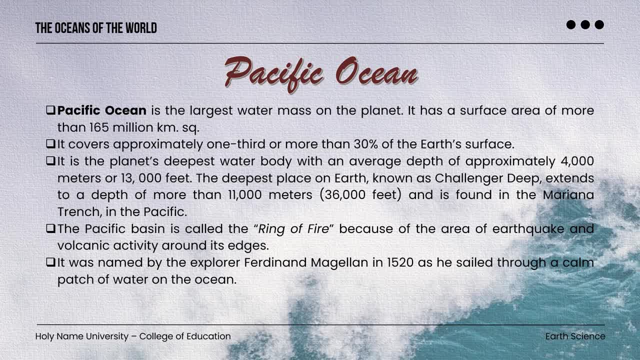 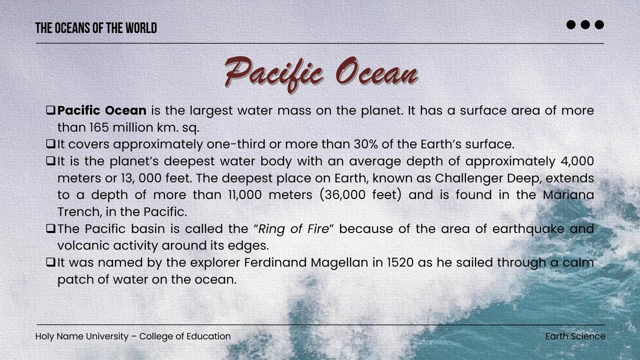 So Pacific Ocean comes from the word pacify, which means peaceful, So maunang di nga nila ni Ferdinand Magellan og Pacific So very interesting. Karoon pa pood ko na kaibaw ani, And I don't know if kaibaw na ba pood mo ani, but yeah. 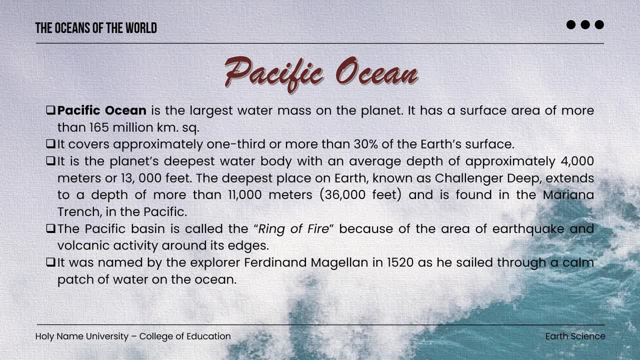 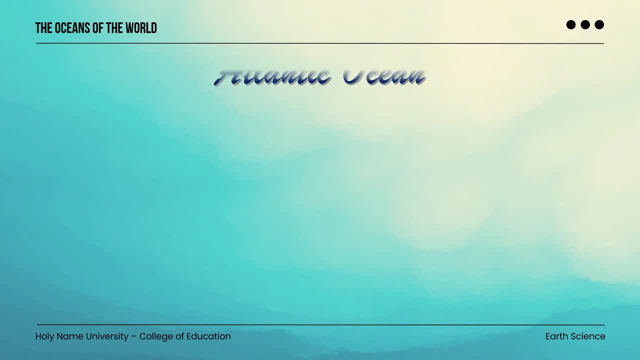 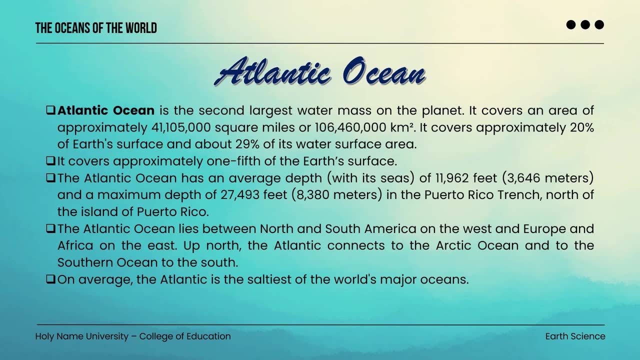 It's kind of new to me. So the next ocean that we will be talking about is the Atlantic Ocean. Atlantic Ocean is the second largest water mass in the planet. It covers an area of approximately 41,105,000 square miles, or 106,460.. 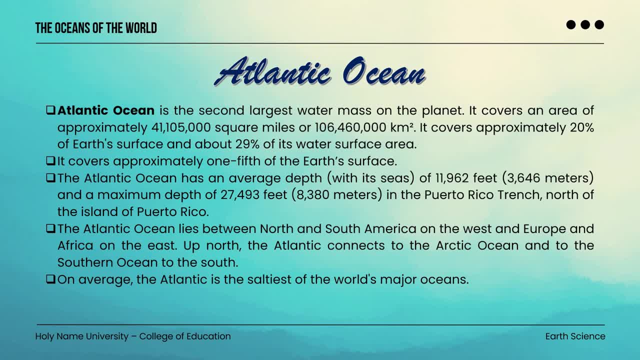 I'm sorry, 106,000.. 460,000 kilometers squared, It covers approximately 20% of Earth's surface and about 29% of its water surface area. It covers approximately one-fifth of the Earth's surface. The Atlantic Ocean has an average depth of 11,962 feet or 3,646 meters, and a maximum depth of 27,000.. 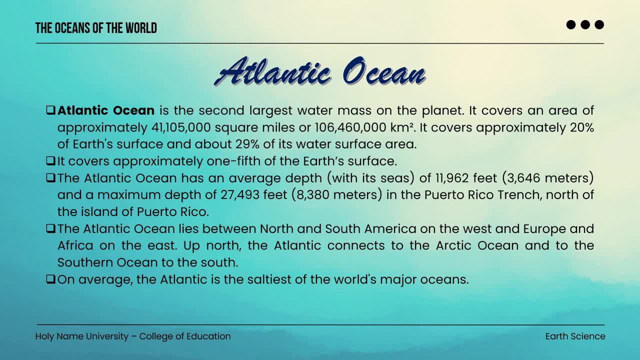 493 feet In the Puerto Rico Trench, north of the island of Puerto Rico. The Atlantic Ocean lies between North and South America on the west and Europe and Africa on the east. Up north, the Atlantic connects to the Arctic Ocean and to the southern Ocean, to the south. 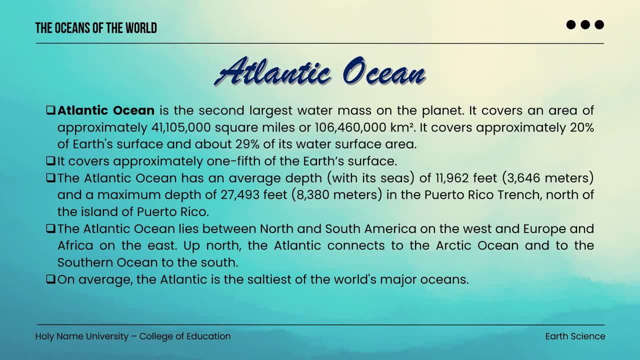 On the average. the Atlantic Ocean is the saltiest of the world's major oceans. This is because the salinity of of the surface waters in the open ocean ranges to 33 to 37 parts per thousand by mass and varies with latitude and season. when we say salinity, that is the 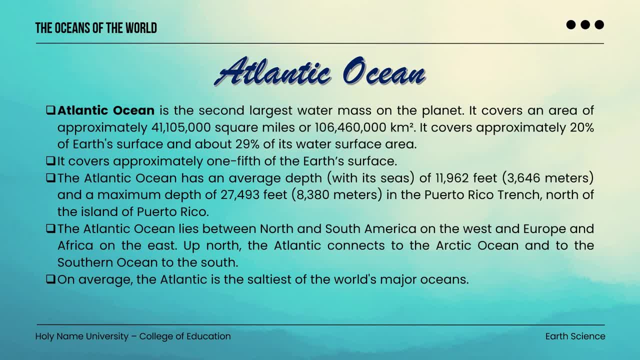 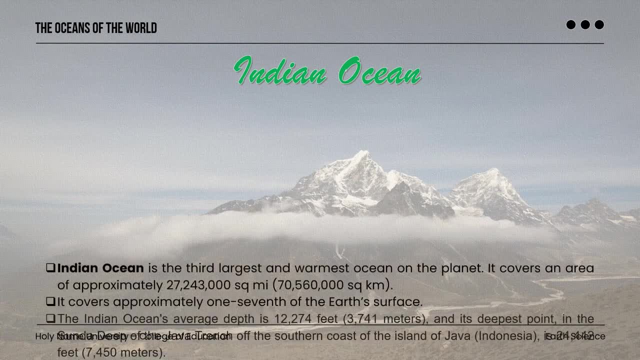 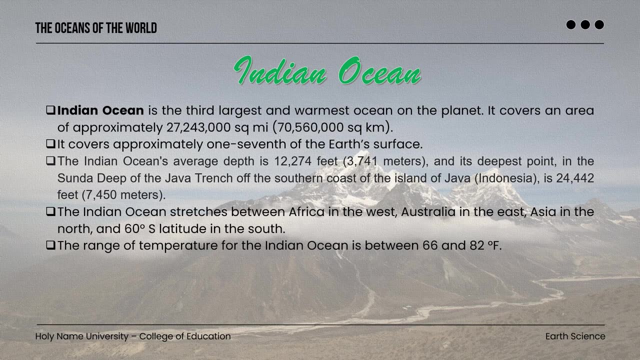 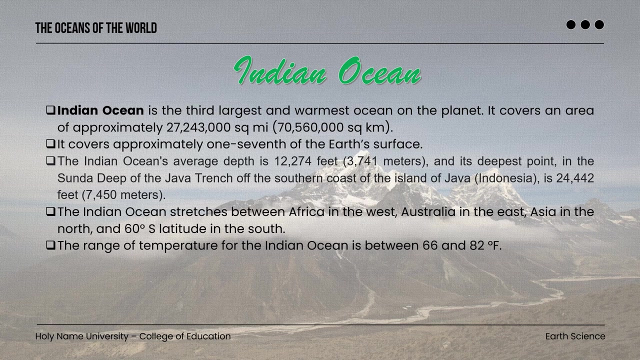 concentration of salt in water. so next up we have Indian Ocean. Indian Ocean is the third largest and warmest ocean and the planet. that covers an area of approximately twenty seven million two hundred forty three thousand square miles, or seventy million five hundred sixty thousand square kilometers. it covers approximately 1, 7 of the Earth's. 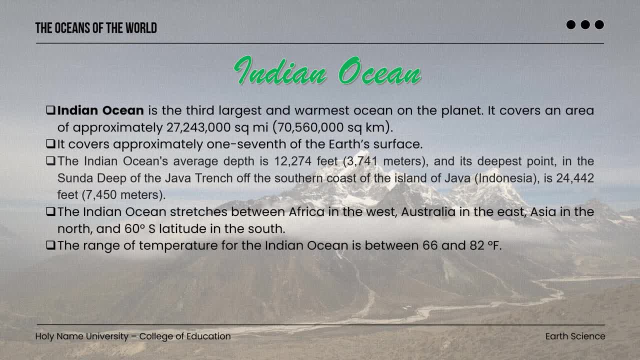 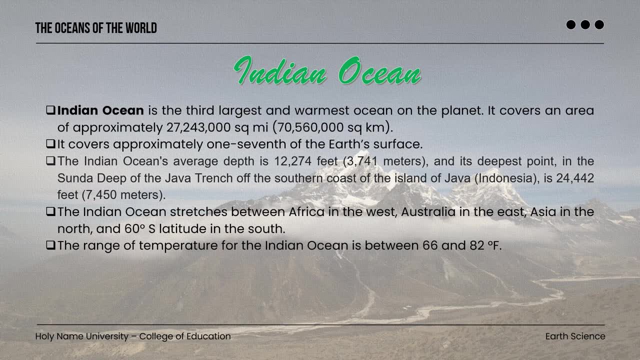 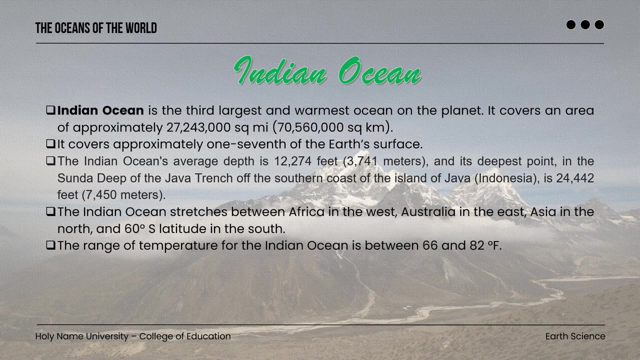 surface. the Indian Ocean's average depth is twelve thousand two hundred seventy four feet, or just equal to three thousand seven and forty one meters of, And its deepest point in the Sunda Deep of the Java Trench, off the southern coast of the island of Java in Indonesia, is 24,442 feet, or just equal to 7,450 meters. 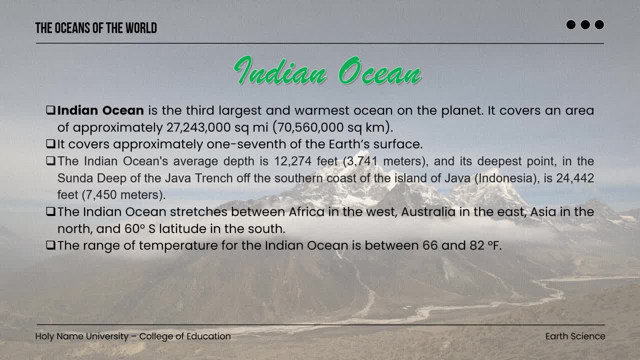 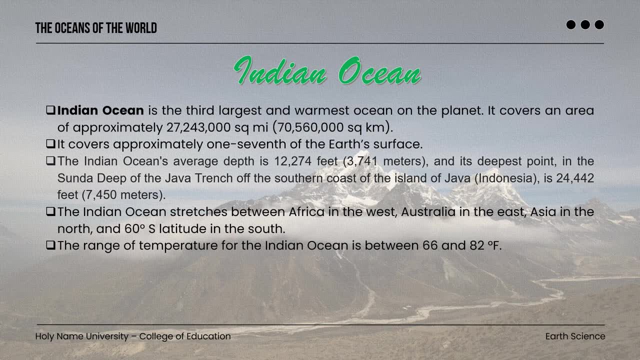 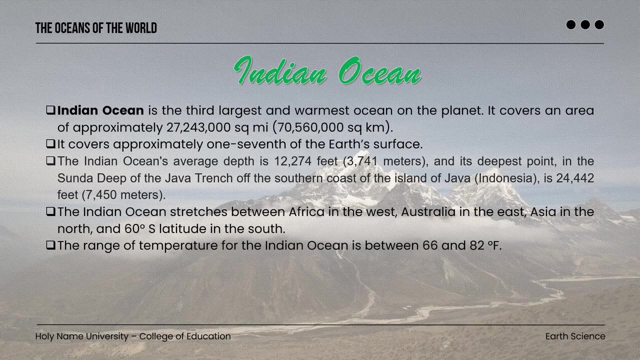 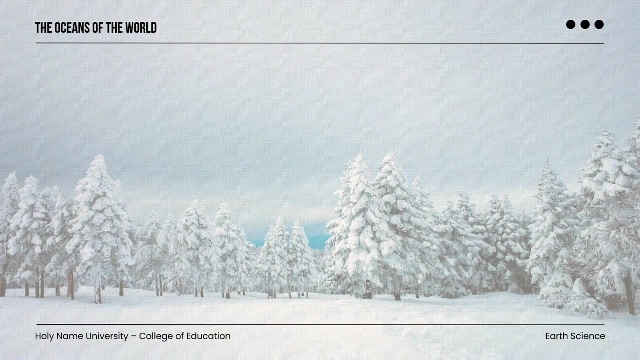 So the Indian Ocean stretches between Africa in the west, Australia in the east, Asia in the north and 60 degrees south latitude. in the south, The range of temperature for the Indian Ocean is between 66 and 82 degrees Fahrenheit. The next ocean that we will be tackling about is the Southern Ocean. 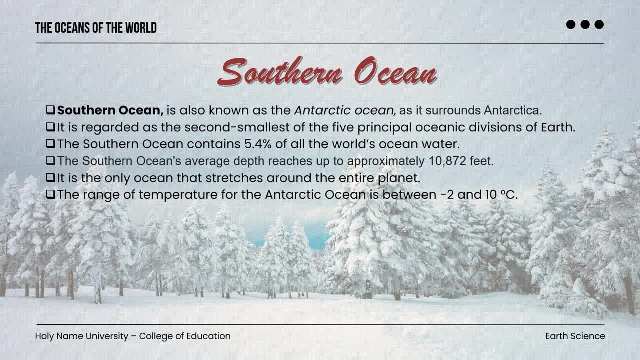 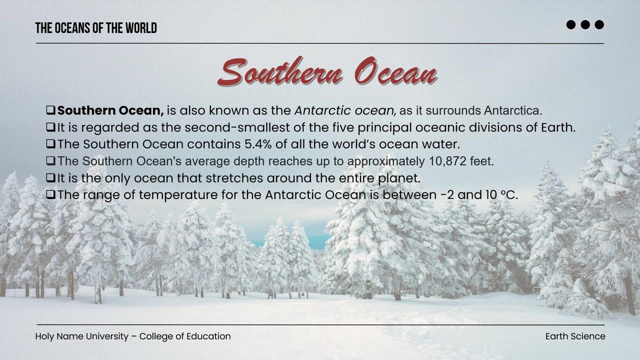 Southern Ocean is also known as the Antarctic Ocean, as it surrounds Antarctica. It is regarded as the second smallest of the five principal oceans. It has the highest dynamic divisions of the Earth. The Southern Ocean contains 5.4% of all the world's ocean water. 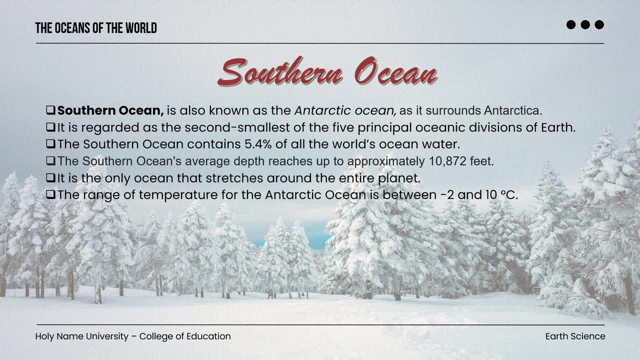 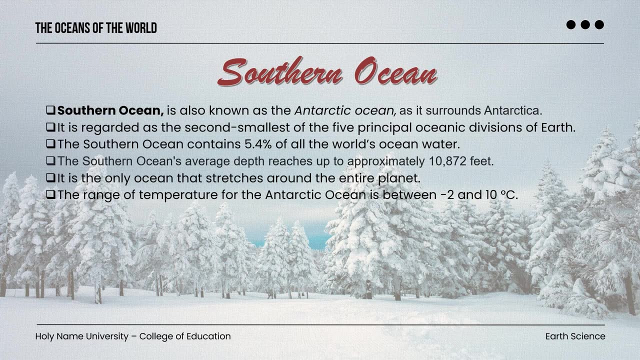 The Southern Ocean's average depth reaches up to approximately 10,872 feet. It is the only ocean that stretches around the entire planet, because it connects all major ocean basins except the Arctic. So the range of temperature for The Antarctic Ocean is between negative 2 and 10 degrees Celsius. 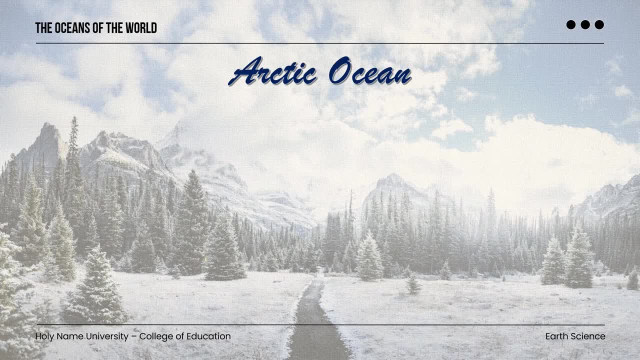 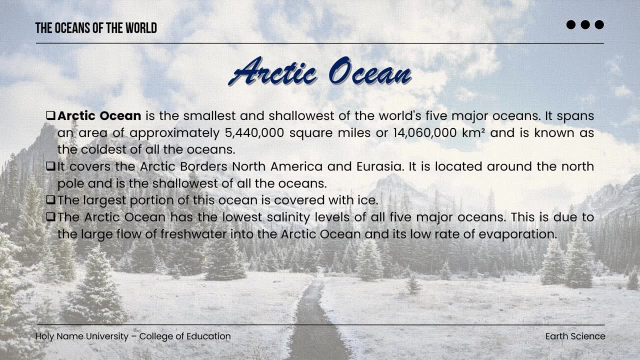 And we have, last but not the least, we have Arctic Ocean. So the Arctic Ocean is the smallest and the shallowest of the world's five major oceans. It spans an area of approximately 5,440,000 square miles, or just equal to 14,060,000 kilometers squared, and is known as the coldest of all the oceans. 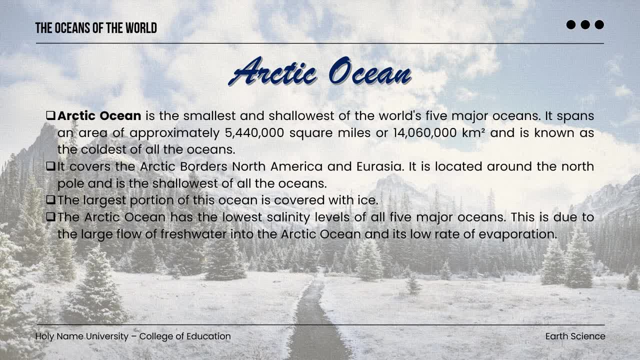 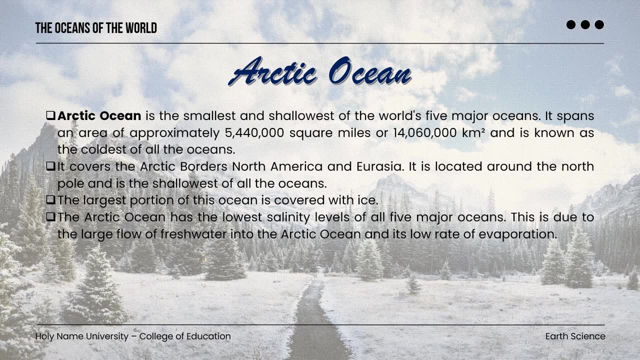 So, though, the Southern Ocean, or the Antarctic Ocean has also ice or snow on it, but the ocean that is considered as the coldest among the five is the Arctic Ocean, So it covers the Arctic borders, North America and Eurasia. It is located around the North Pole and is the shallowest of all the oceans. 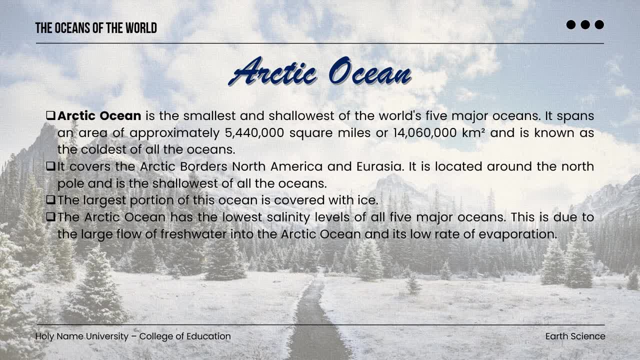 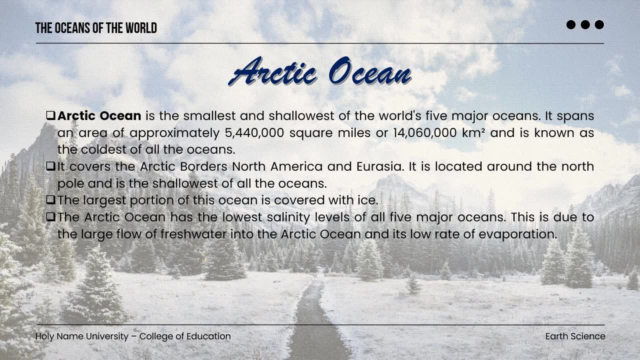 The largest portion of this ocean is covered with ice. The Arctic Ocean has the lowest salinity levels of all five major oceans. This is due to the large flow of fresh water into the Arctic Ocean and its low rate of evaporation. So, to sum it up, we have five major oceans. 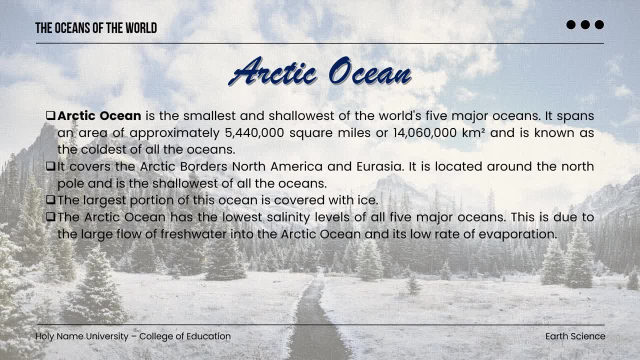 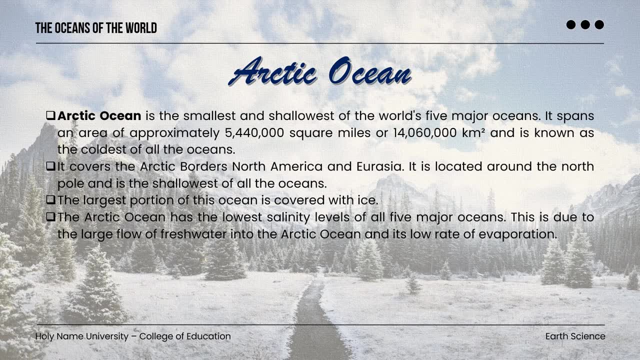 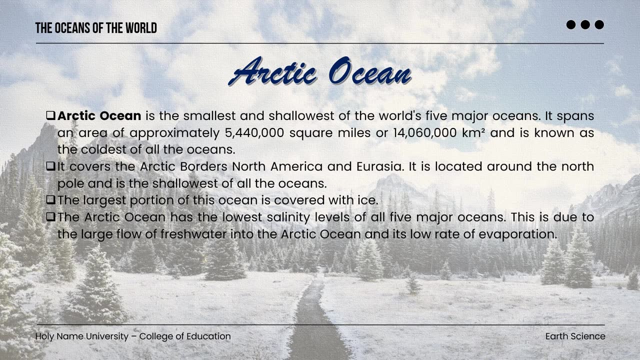 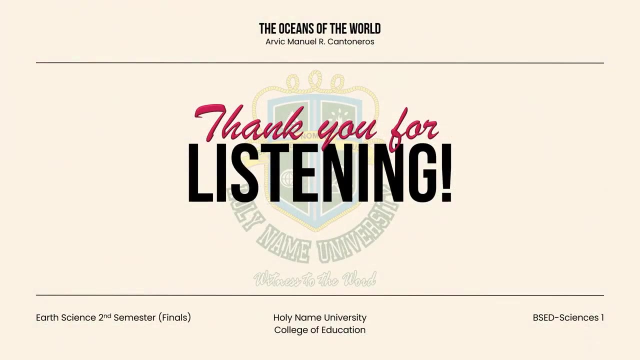 And the largest one is the first. We have Pacific Ocean, The next is we have Atlantic Ocean, Indian Ocean, The Southern or the Antarctic Ocean And lastly, we have the Arctic Ocean. And that concludes my presentation for the oceans of the world. 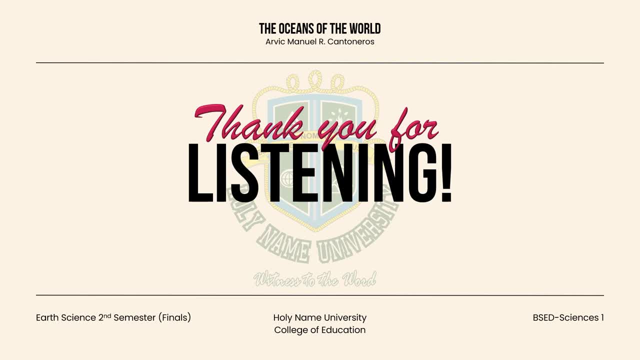 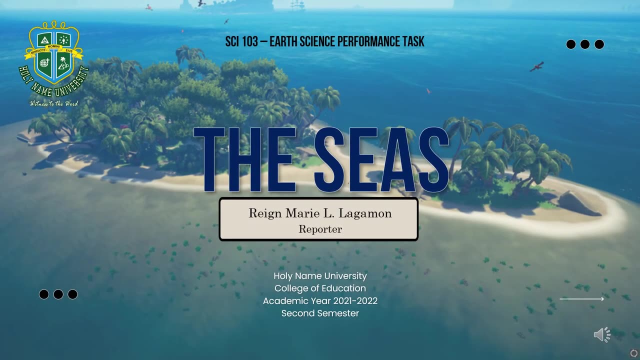 So the next reporter would be Miss Rain Marie Lagamon, And she will be tackling about the seas. So that would be all. Thank you so much for listening and God bless us all. Hi everyone, My name is Rain Marie Lagamon and I'm here to discuss about the seas. 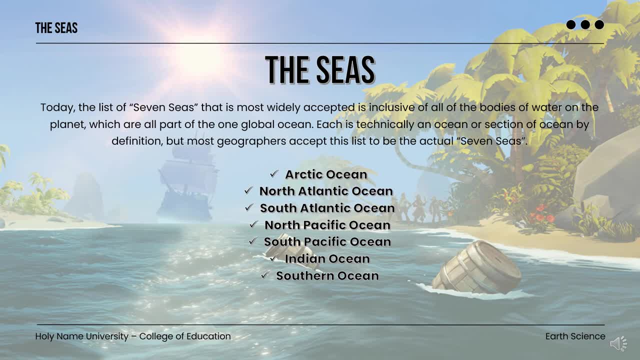 The Seas. Today, the list of seven seas That is most widely accepted is inclusive of all the bodies of water on the planet, Which are all part of the one global ocean. Each is technically an ocean or section of ocean by definition, But most geographers accept this list to be actual seven seas. 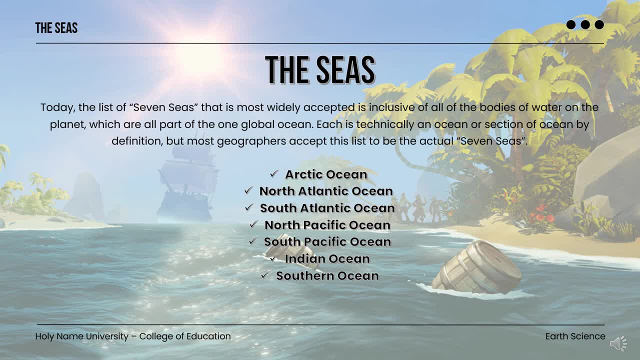 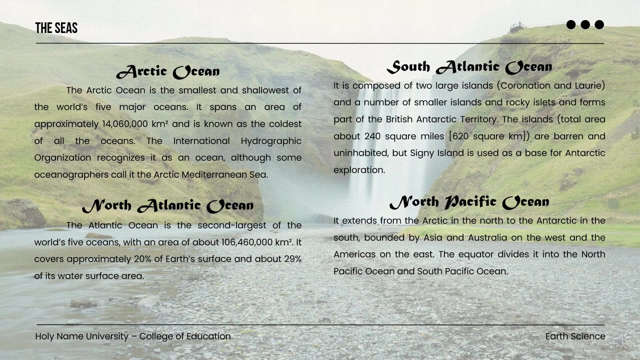 So here's the seven seas. The first one is Arctic Ocean, North Atlantic Ocean, South Atlantic Ocean, North Pacific Ocean, South Pacific Ocean, Indian Ocean And the Southern Ocean, The Arctic Ocean. The Arctic Ocean is the smallest and swallowest of the world's five major oceans. 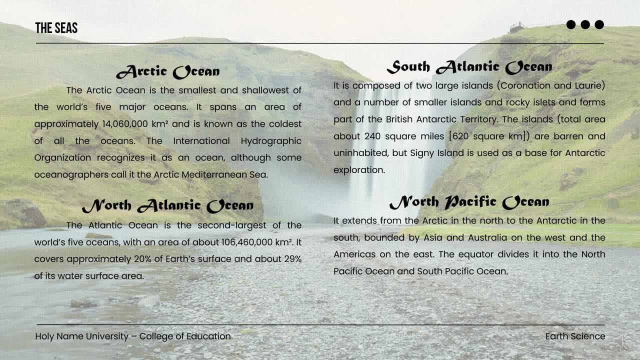 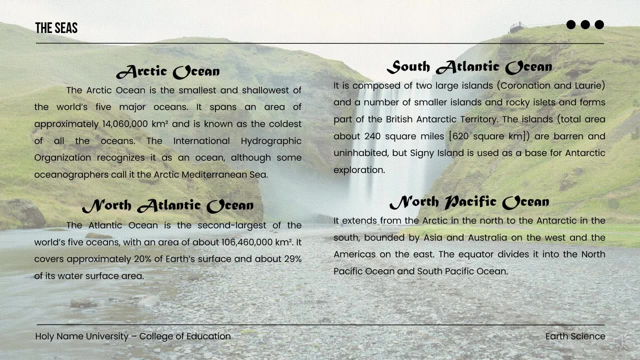 It spans an area of approximately 1,000 km and is known as the coldest of all the oceans. The International Hydrographic Organization recognizes it as an ocean, Although some oceanographers call it the Arctic Mediterranean Sea. The second one is the North Atlantic Ocean. 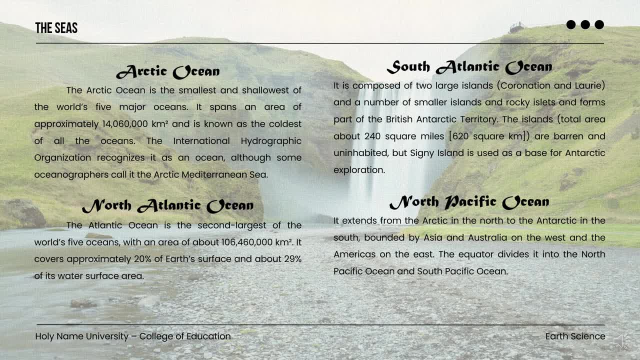 The Atlantic Ocean is the second largest of the world's five oceans, With the largest ocean in the world. The Arctic Ocean is the second largest of the world's five oceans. With an area of about 106,460,000 km, it covers approximately 20% of Earth's surface. 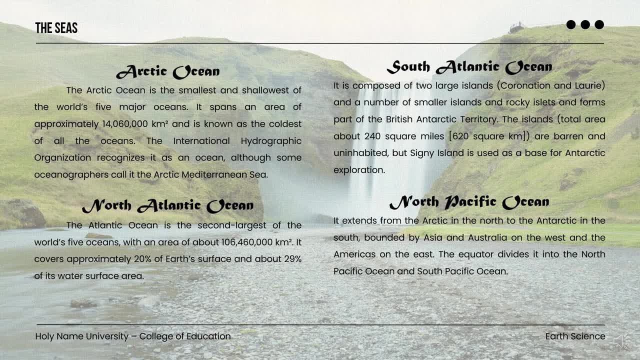 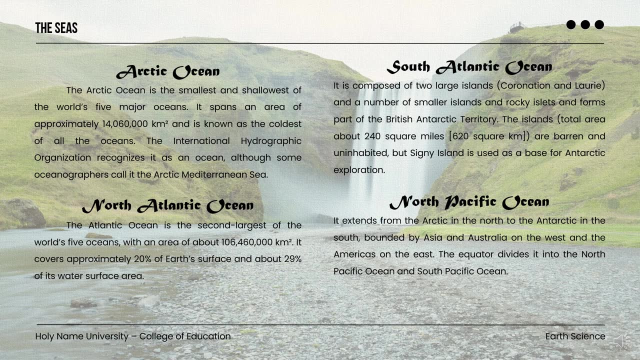 and about 29% of its water surface area. The third one is South Atlantic Ocean. It is composed of two large islands, Coronation and Lowry, and a number of smaller islands and rocky islands. The North Atlantic Ocean is a Craig- Grade islands islets and forms part of the British 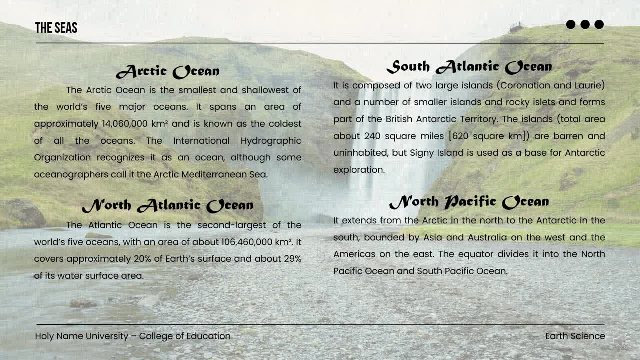 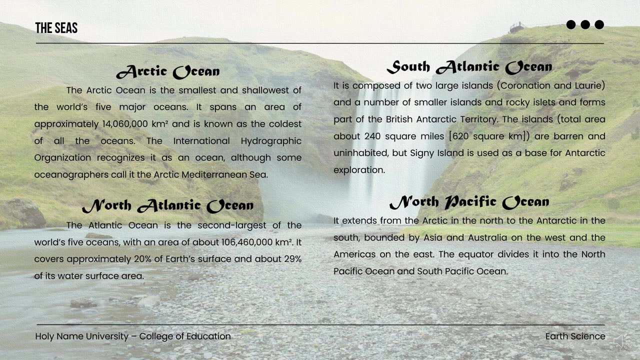 Antarctic Territory. The island's total area about 240 sq miles, 620KM square, Are barren and uninhabited, but a sunny island is used as a base for Antarctic exploration. The fourth one is the North Pacific Ocean. It extended around 3,000Serpentines. 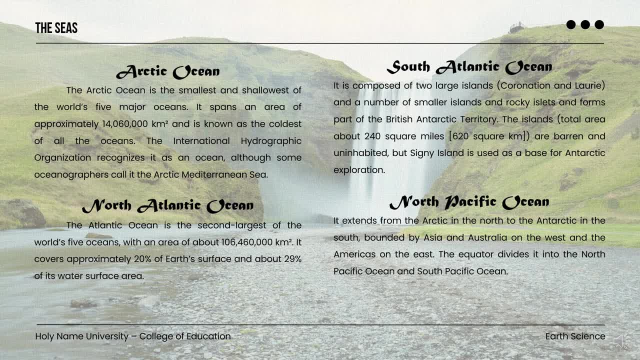 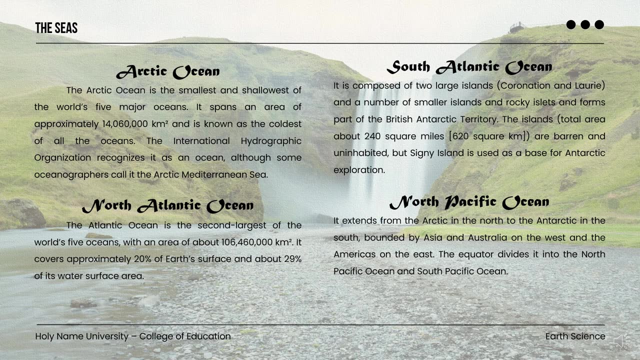 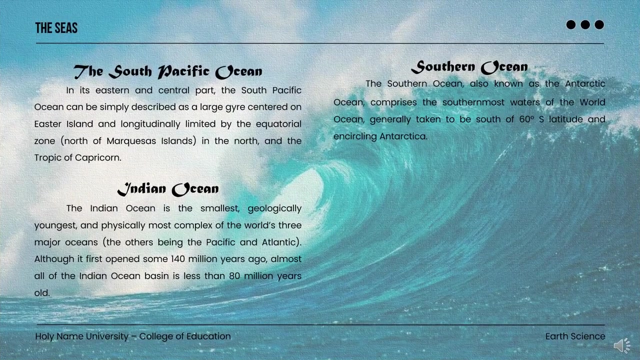 It extends from the Arctic in the north to the Antarctic in the south, bounded by Asia and Australia on the west and the Americas on the east. The equator divides it into the North Pacific Ocean and South Pacific Ocean, The South Pacific Ocean In its eastern and central part. the South Pacific Ocean can be simply described as a large centered on an eastern island and longitudinally limited by the equatorial zone north of Marquesas Islands, in the north and the Tropic of Capricorn.